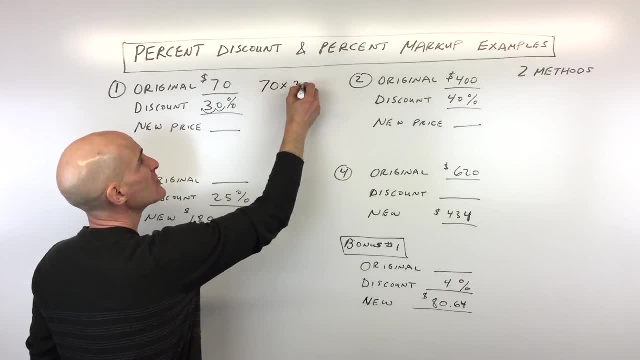 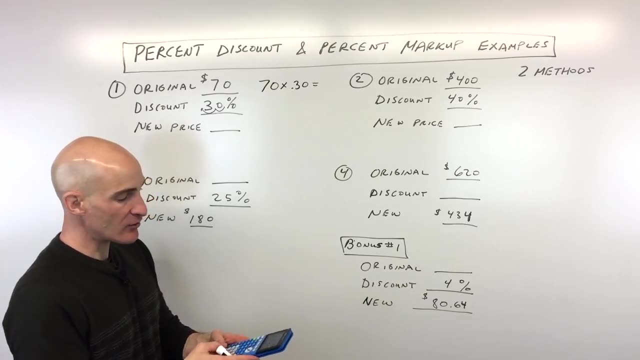 that decimal point two places to the left. So that's going to be 0.30.. And if we multiply those together, we can use a calculator. You can do this by hand. We're just going to multiply those together 70 times 0.30, that comes out to $21.. So what that means is that you're saving $21,. 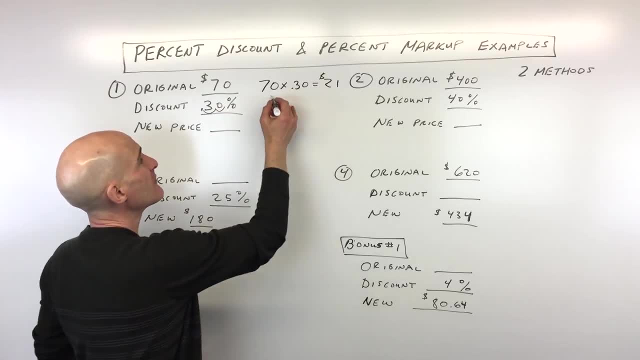 right, But that means you're going to have to take away the $21 from 70.. So 70 minus 21 equals how much? $49, right, So that's going to be your new price. Now, that's one method I'm going to. 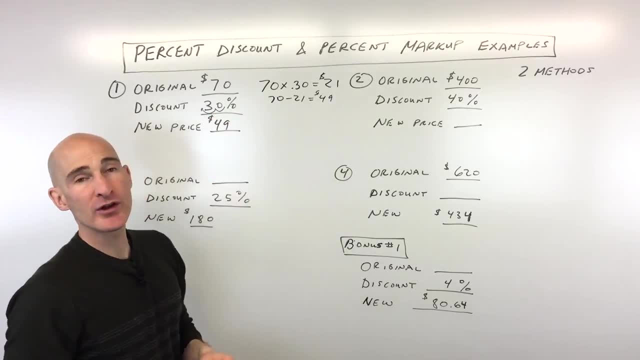 show you a quicker method now, And this quicker method is, instead of focusing on what you're saving, focus on what you're paying. So what percentage would you be paying if it's 30% discounted or 30% off? Well, you'd be paying 70%, right? So what you can do is you can jump. 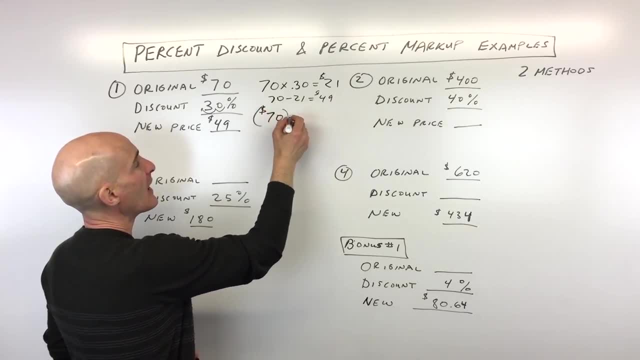 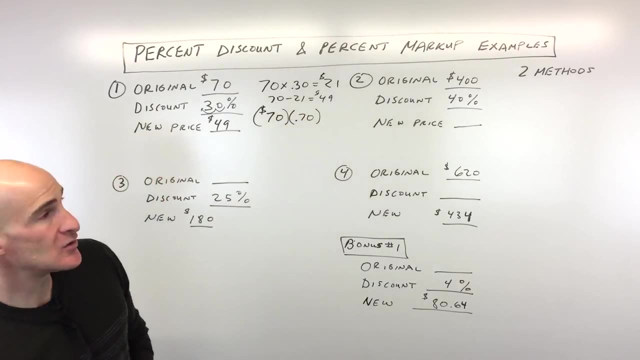 right to $70.. And we're going to multiply that by 70%, which 70% as a decimal is 0.70.. I just moved the decimal two places to the left, So now all we have to do is multiply 70 times 0.70.. 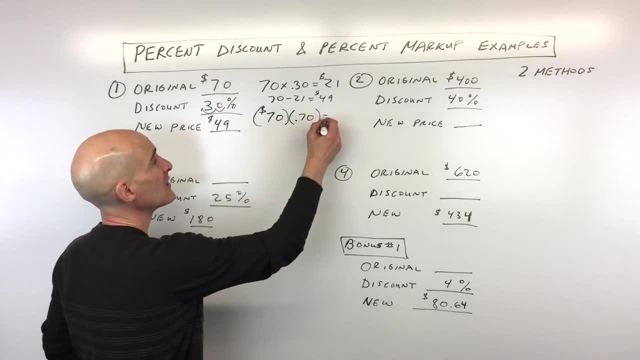 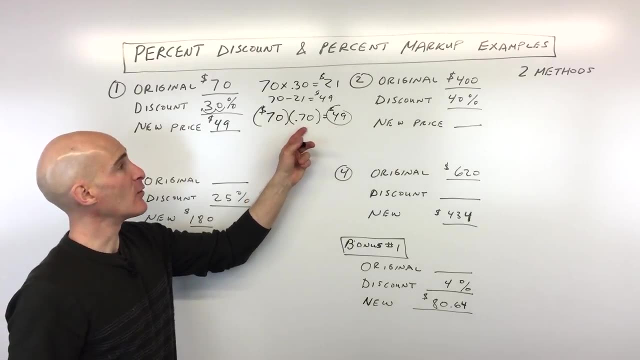 And we're getting $49, which is the exact same thing that we got in method one above. The only difference here is a little bit quicker. We did it in one step because we focused on what we're paying And we figured out what that percentage was by taking. 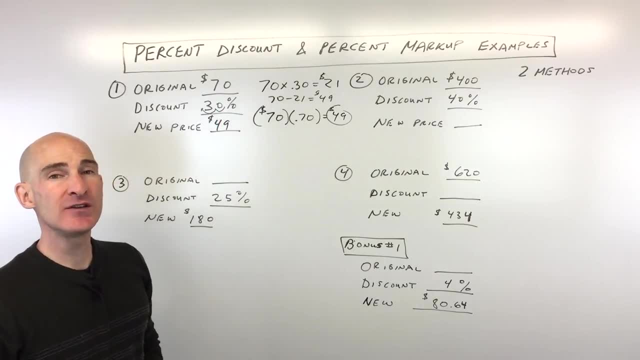 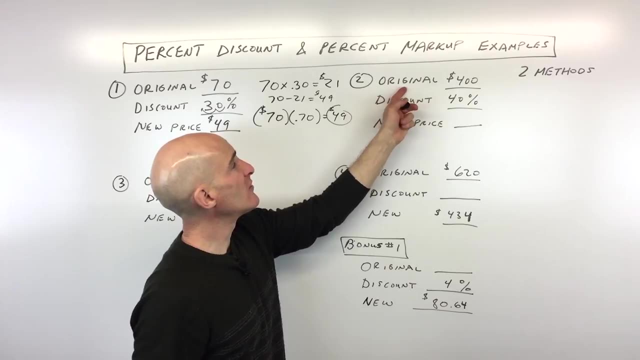 100% minus 30%. Okay, let's look at another example. See if you can do this one on your own. If you want, you can pause the video and go ahead and then check it back with me here. So let's see. So number two we've got. the original price of an item is $400.. The discount is 40%. 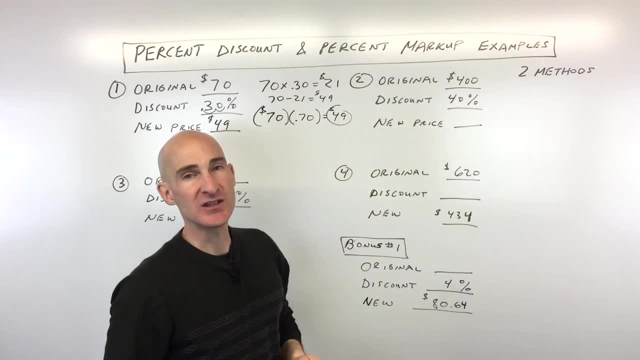 So it's like 40% off, And now we want to find out what the new price is. So you can use either one of the methods. I'll do both methods for this one, But let's see the next one. I'll just pick. 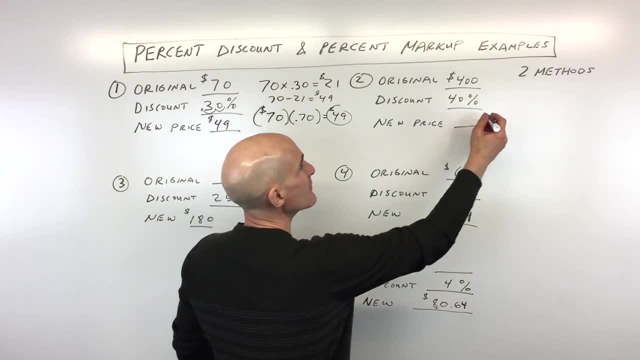 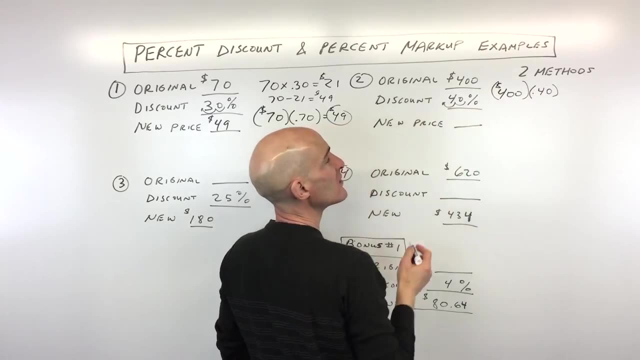 one of the methods. So here the discount is 40%. So let's see what we're going to save. So we're going to take $400.. We're going to multiply by 40%, which is 0.40 as a decimal. Okay, so move. 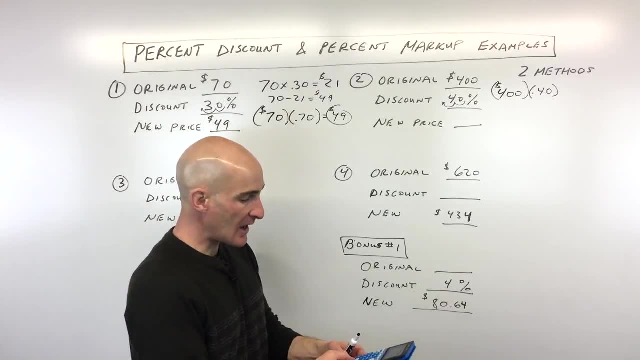 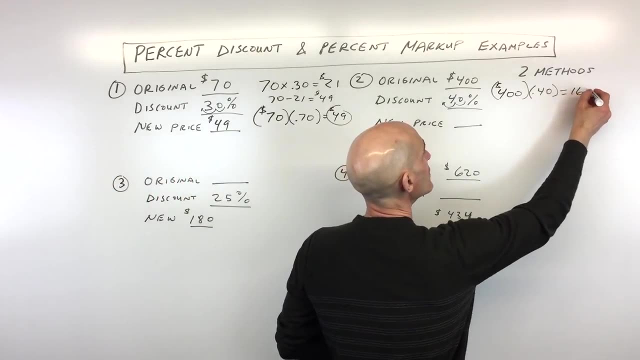 that decimal two places to the left. And if we do that- you can do that by hand or you can do it on a calculator- We're getting $160, right? So that means that you're going to be saving $160.. So we 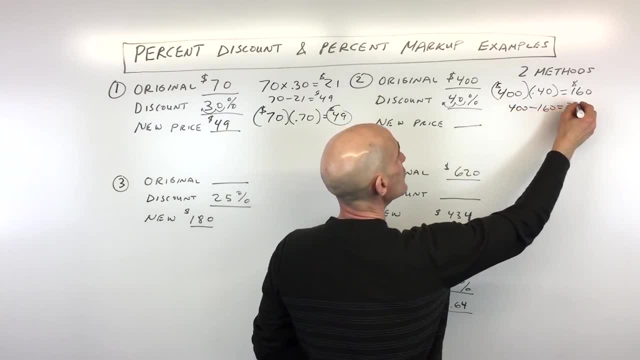 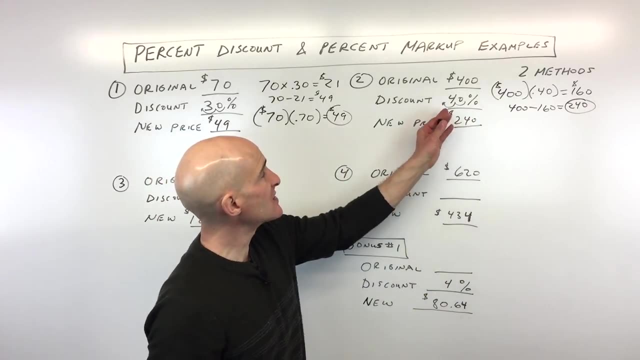 have to take the $400 minus $160, which means that you're going to be saving $160.. So that means that you're going to pay the new price of $240.. Now method number two. let's just say, instead of taking 40% off, let's just say that we're going to focus on what you're going to pay, which is 60%. 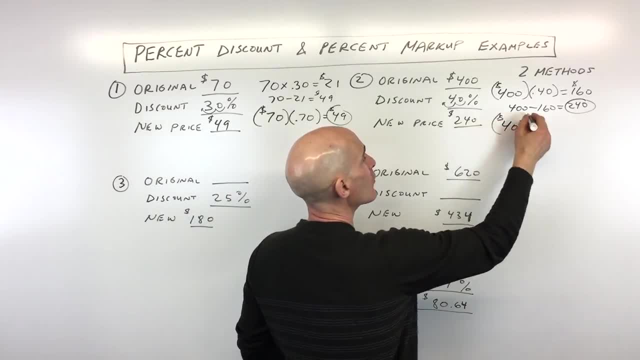 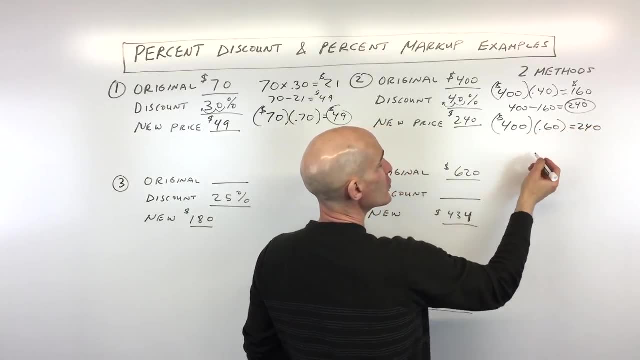 right. So we're just going to take the $400.. We're going to multiply by 60%, which is 0.60.. And if you do that on a calculator, you're going to get 240, or you can do it by hand, Okay, so 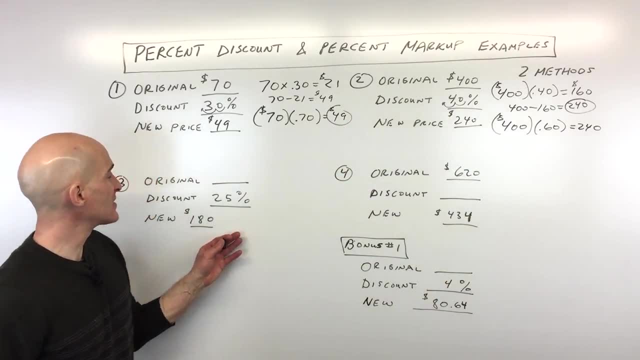 that's number two. So let's jump into number three. I'm just going to pick one of the methods for this one. So here it's a little bit more challenging. but it's a little bit more challenging because we don't know what the original price is. We know what the new price is and we know what. 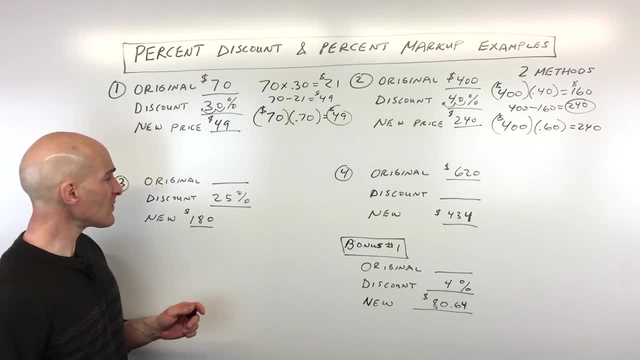 the discount is. So how do we solve a problem like this? Well, there's a couple different ways to do it. I'm going to write an equation. So what I'm going to do is I'm going to say, hmm, that original. 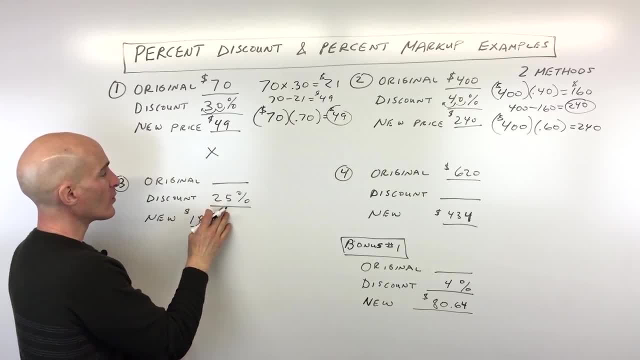 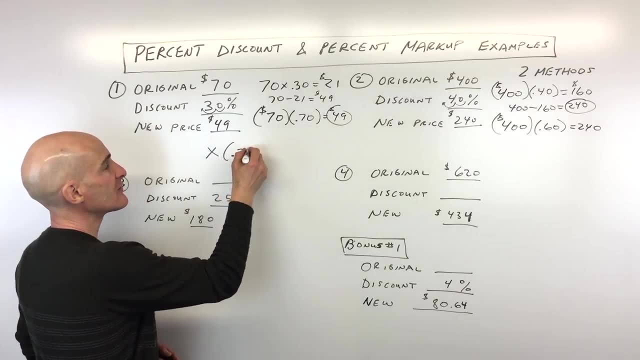 price. let's call that X, since we don't know what it is. Now. it's being discounted by 25%, but that means you're actually going to pay 75%, right? 75% is really 0.75 as a decimal. 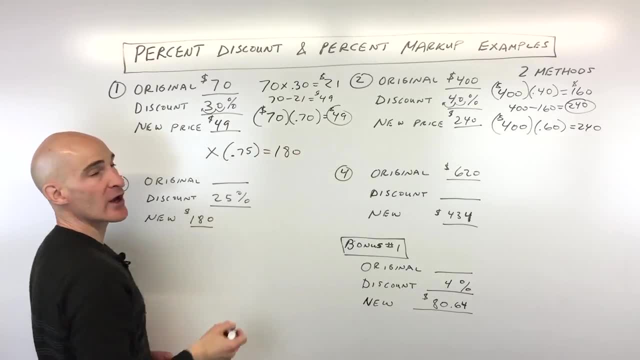 And the answer to that is going to be the new price, $180.. So just to go over real quick again, the starting price, which we don't know, X times the amount that you're going to pay, equals the new price. So now all we have to do to solve for X is to divide both sides. 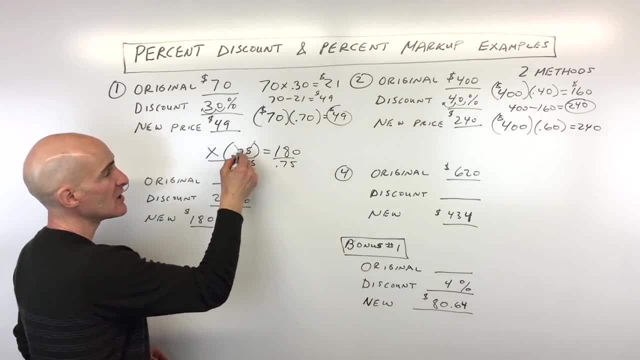 by 0.75.. See how these are multiplied together. We're doing the inverse, which is to multiply both sides, And let's just go to the calculator. Let's see what that is: 180 divided by 0.75.. Okay, 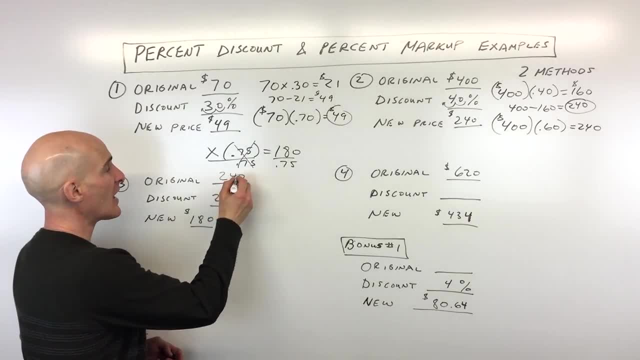 we're getting $240.. And you got it. Now, if you want to check your work, you of course can. You just have to take $240 times 0.25.. Okay, and that's going to be how much that you're saving. Subtract that from the 240,. 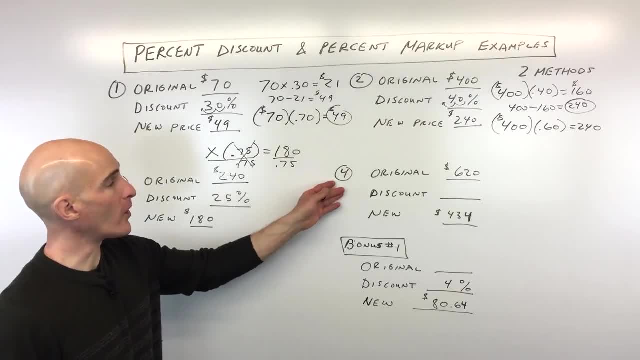 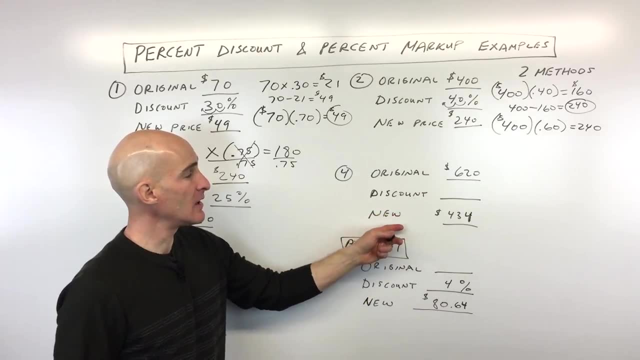 and you're going to get 180.. Okay, let's do another example. So, number four: we've got the original price of $620.. But now we don't know what the discount is. We don't know that percent discount And we know the new price is $434.. So what do you think for this one? How? 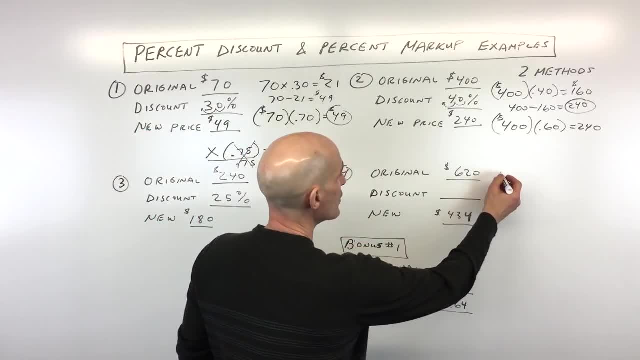 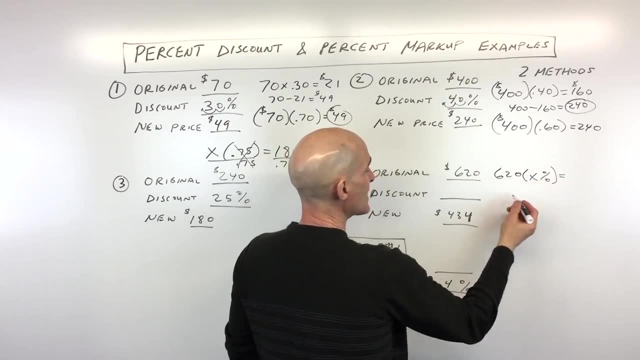 can we approach this one? Well, let's go ahead and write an equation. So we're going to start off with the $620.. And we're going to multiply by, let's just say, X percent, Okay, And then that's going to give us the new price, $434.. Now, this X percent, the way I've set this up. 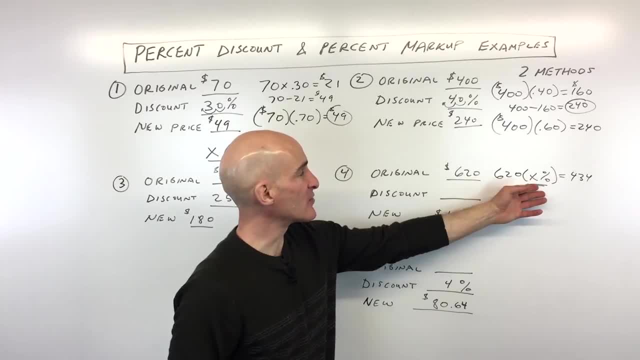 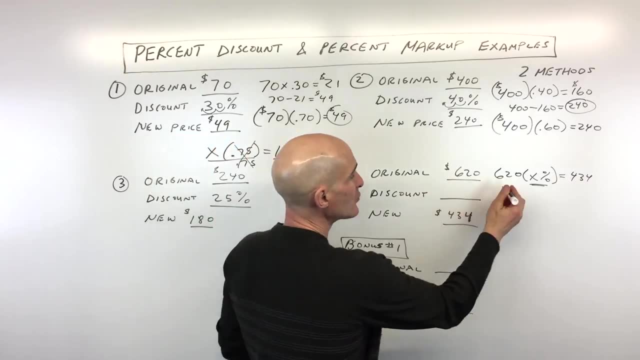 this is going to be the percentage that you pay, right? So you're paying that percent of the original price and that's your new price. So keep that in mind. So now, what we're going to do is we're going to divide both sides by 620.. Okay, and now we're left with X. Okay, and let's see. 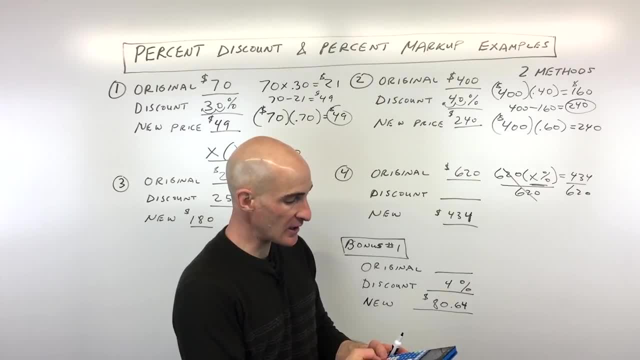 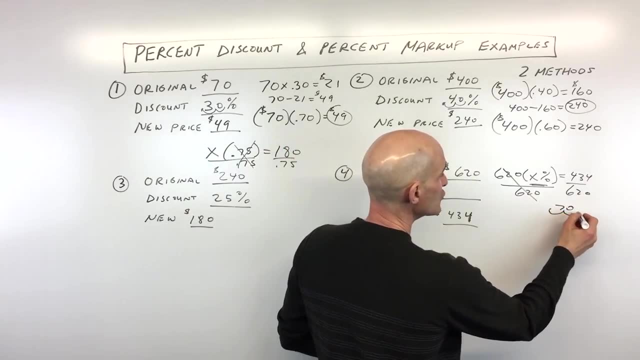 what that comes out to. So we've got 434 divided by 620.. It's coming out to 0.70.. As a percentage, we have to move that decimal two places to the right. That's 70%. Now that means 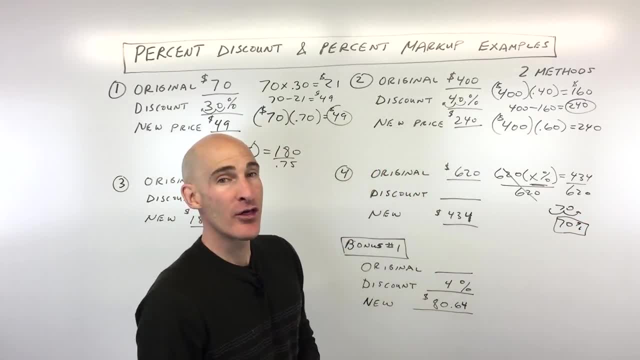 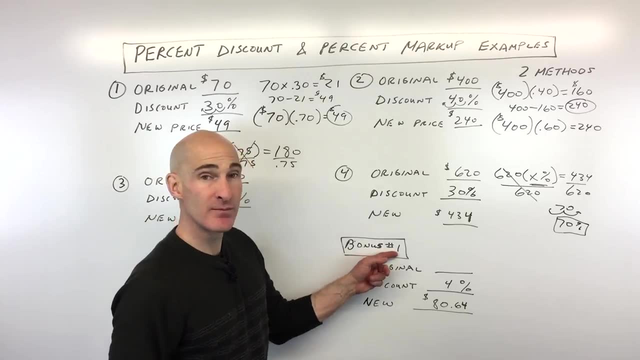 you're paying 70%, But what's the discount? 30%, right? So that's going to be our discount. Okay, now we've got one additional problem. If you want, I call this bonus number one. Go ahead and see if. 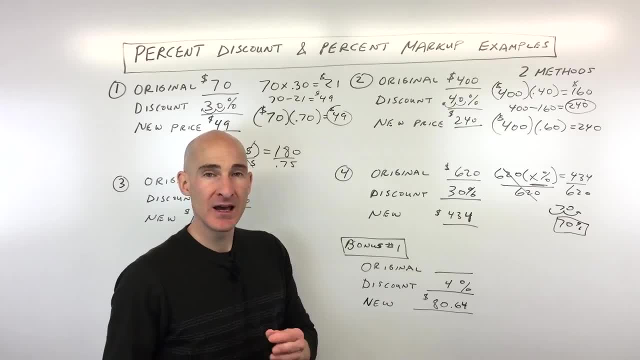 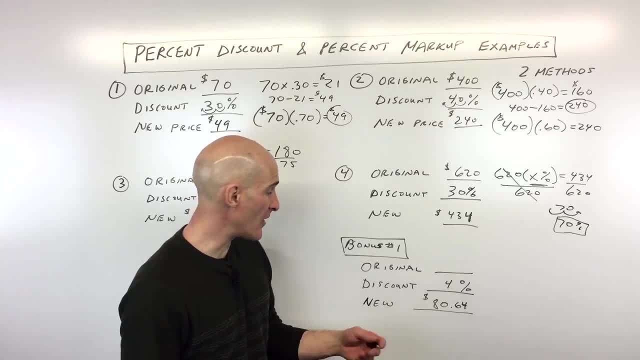 discount percentage is 4%. So 4% off, And the new price is $80.64.. So go ahead and try that one on your own. I'm going to wipe the whiteboard down real quick And we're going to do the percent. 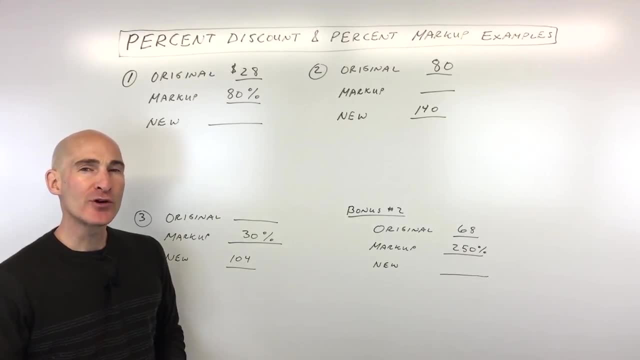 markup problems next. Okay, now we're going to talk about percent markup, So let's go through some examples together. I'll show you the two different methods for solving these types of problems. So let's say your original amount is $28.. And then the markup is 80% And you want to find out what the new price is going to be. So let's say you're on the right track And you want to find out what the new price is going to be. So say, for example, a store you know they're. 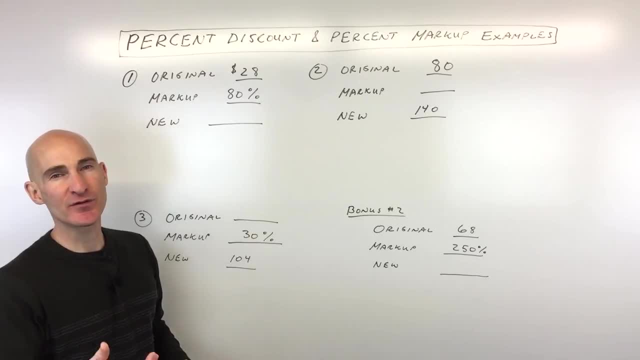 getting in merchandise, they're marking it up, selling it to the customer for additional amount so that they can make a profit, right? So there's two different ways to do this. The first way is you would take the $28 that you're starting with and you would multiply by 80% as a decimal, which. 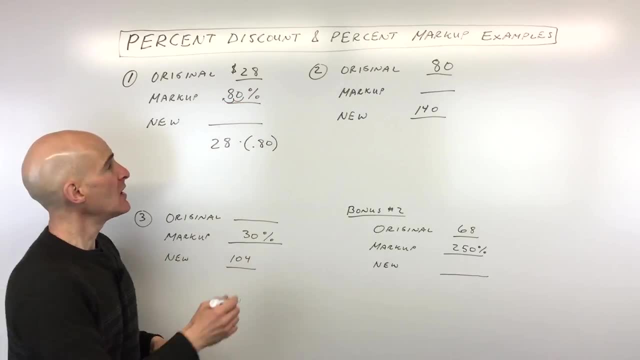 is 0.80.. You want to move that decimal point two places to the left And let's see what that comes out to. So we're going to find out the additional amount that they're going to charge the customer. So that's 28 times 0.80, which comes out to $22.. 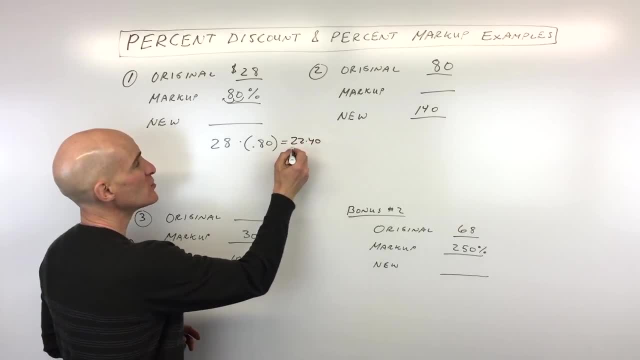 And 40 cents. Now the thing is the $22 and 40 cents. this is the additional amount. we have to add that to the original amount. So I'm going to add the $28. And so now you can see we're getting. 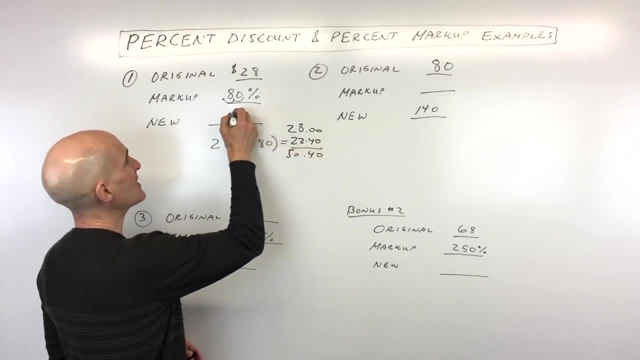 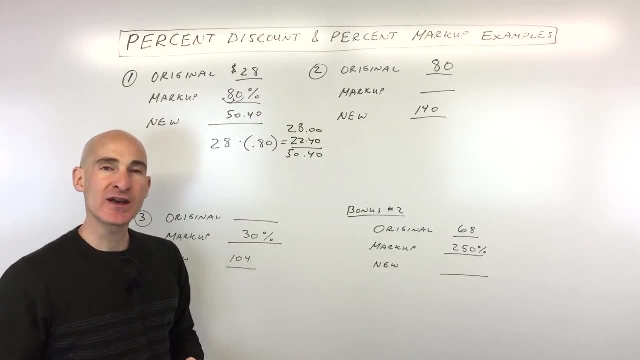 how much this is: $50 and 40 cents. Okay, now there's another way to do this problem. The other way to do it is if they're marking it up by 80%, the customer is actually paying 180%. 100% is the. 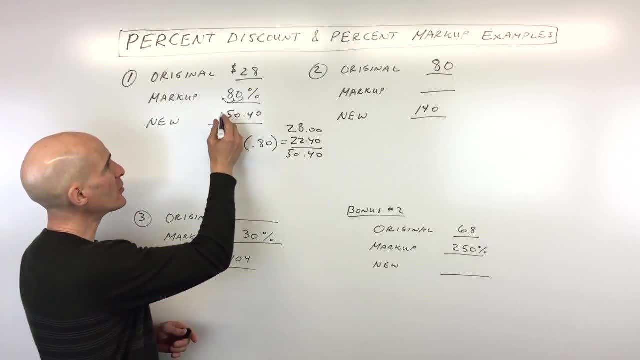 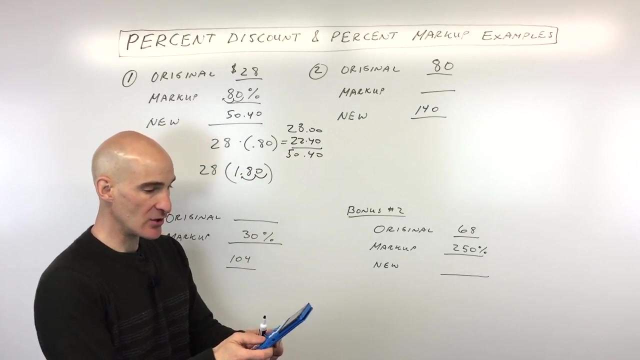 original amount plus an additional 80%. So when you think of 180%, that's actually 1.80.. I just moved that decimal point two places to the left. Now we have to do is take the original amount, the $28 times the 180%, And let's verify that we get the same answer. So 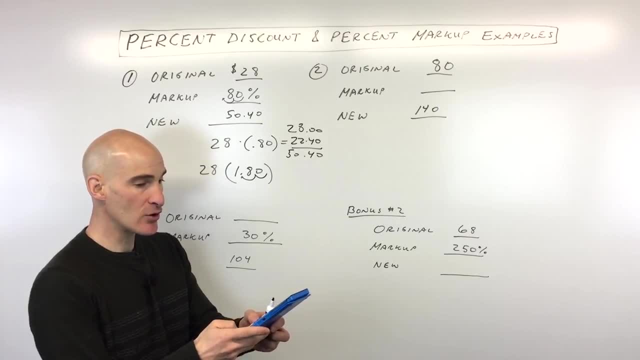 you can do this on your calculator with me if you want. times 1.80.. Again, we get $50 and 40 cents. Okay, let's go to the next example. So each one of these problems is a little bit different than. 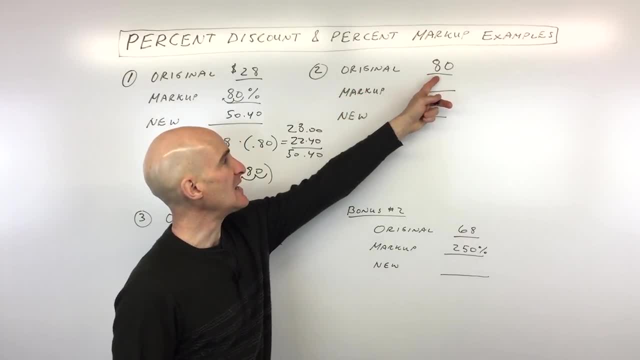 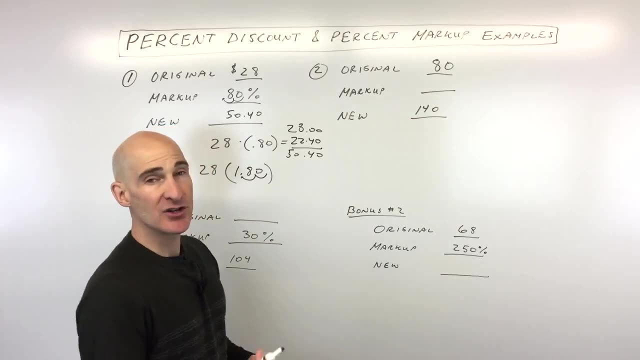 the previous one, So number two: we've got the original amounts 80.. The new amount is 40. But we're wondering: what is that markup percentage? Okay, so what we can do. again, two different methods. One method is: you can see that this is actually increasing in price by $60.. 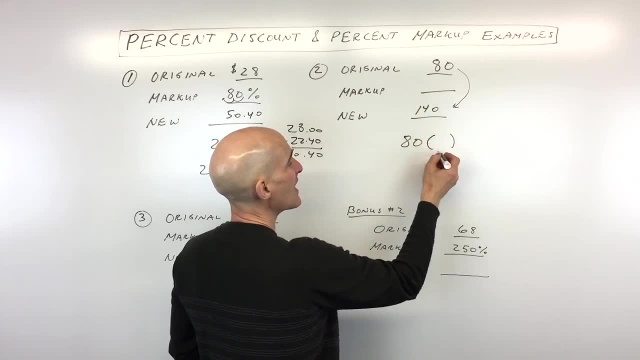 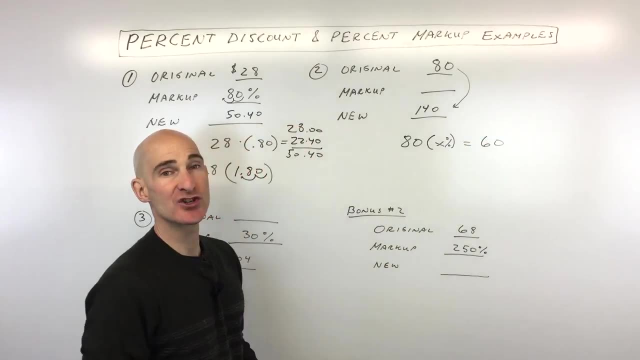 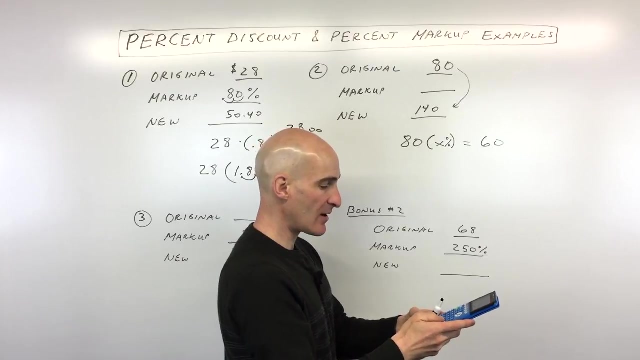 So we'd say $80, the original amount times the percent okay markup equals the additional amount that they're charging the customer, which is an additional $60.. So if we go to the calculator here, I'm going to divide both sides by 80, to get the variable by itself. So 60 divided by 80,. 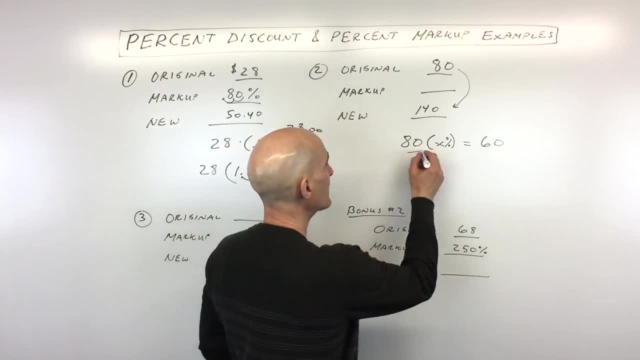 you can see we're getting point seven five. so again, divided both sides by 80, we're getting point seven five. But you see how this is a percentage. we want to move that decimal point two places to the right to convert it back into: 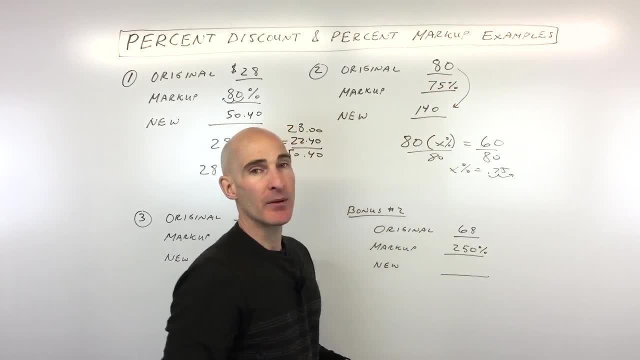 a percentage. So this is actually a 75% markup. Now, the other way to do this problem- and this is the way that I actually like to do it- is I take the $80. And I say 80 times what. so I'll just say: